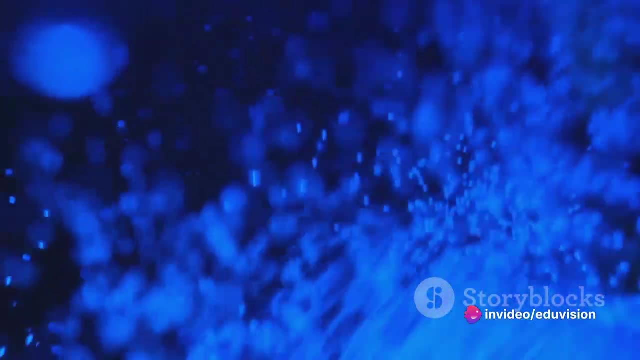 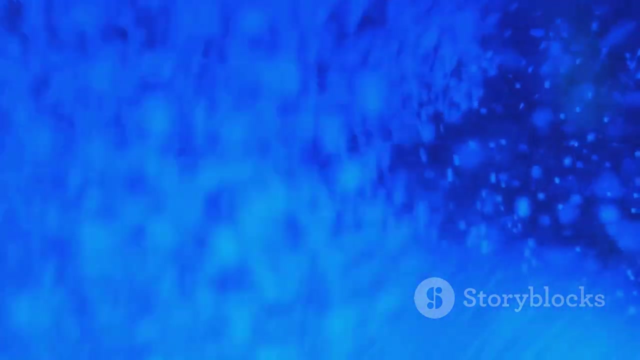 that occurs at temperatures close to absolute zero. You may be familiar with the three commonly known states of matter: solids, liquids and gases. However, science often defies our everyday experiences, introducing us to fascinating phenomena like the Bose-Einstein condensate. 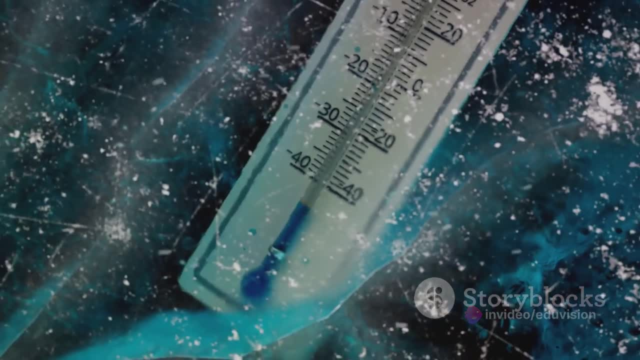 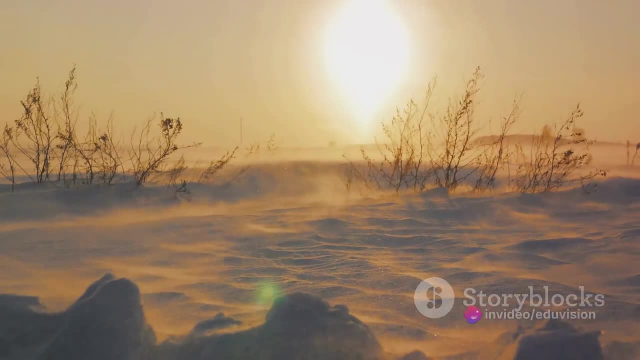 or BC for short. To understand BC, let's first talk about absolute zero. It's the temperature where all classical motion stops, a point so critical that it's hard to believe that it's so cold that nothing could possibly be colder. We're talking about negative 273.15 degrees. 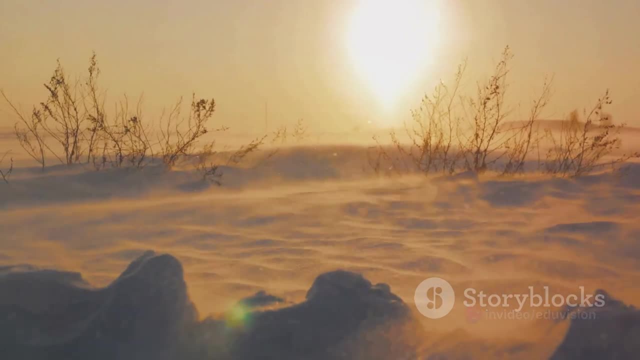 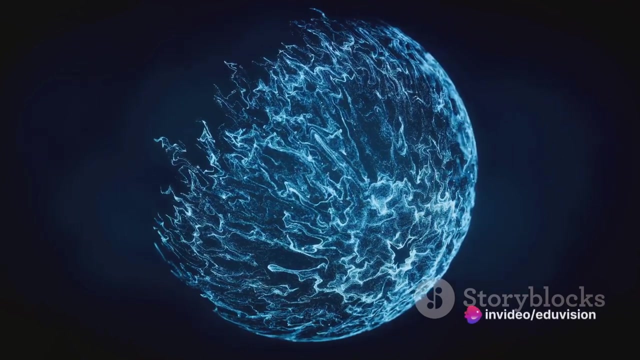 Celsius. That's colder than any natural temperature in the known universe. Now imagine cooling a gas of bosons, a type of particle that likes to stick together. down to these extreme temperatures, The particles slow down to the point where they can't be distinguished from one another. 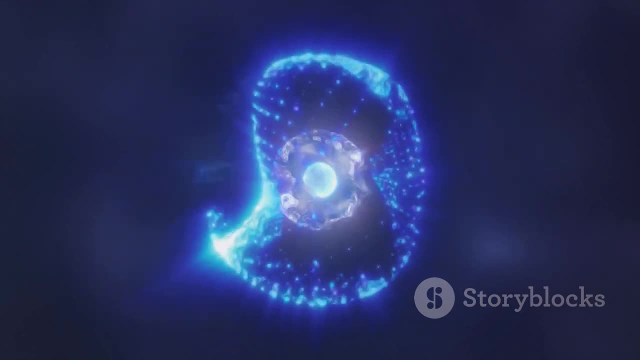 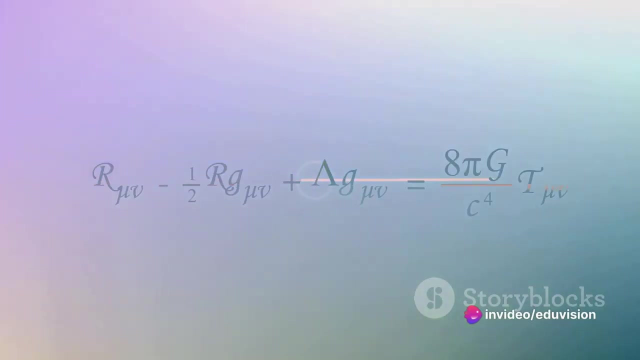 They start to behave as if they were a single particle. This creates a unique state of matter unlike anything we observe in our day-to-day lives. The term Bose-Einstein condensate is named after two brilliant physicists: Satyendra Nath Bose, who first proposed the idea, and Albert Einstein, who expanded upon it. 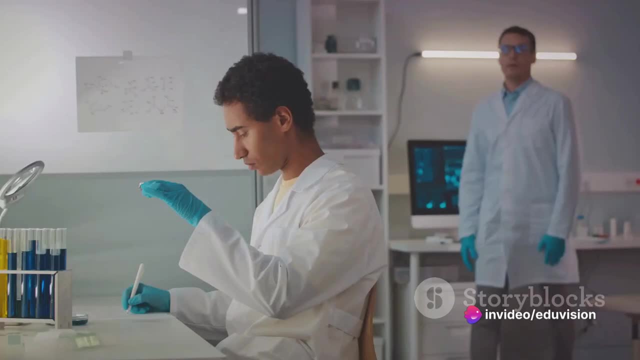 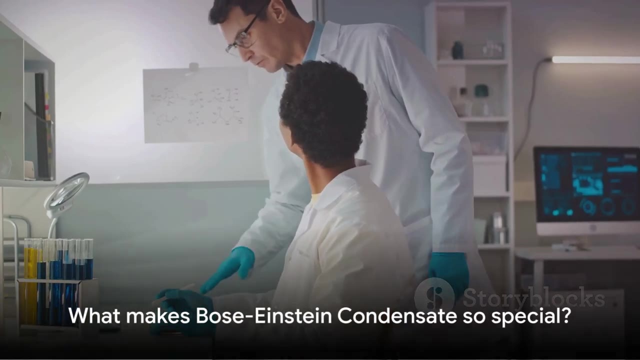 Together. they predicted this peculiar state of matter in the early 20th century, But it wasn't until the late 20th century that scientists were able to create a BC in a laboratory setting. So Bose-Einstein condensate is a super cool state of matter. 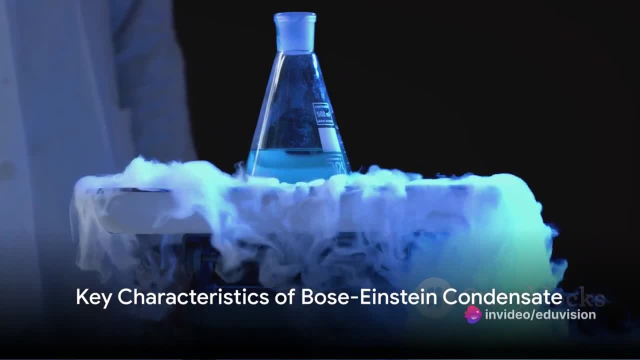 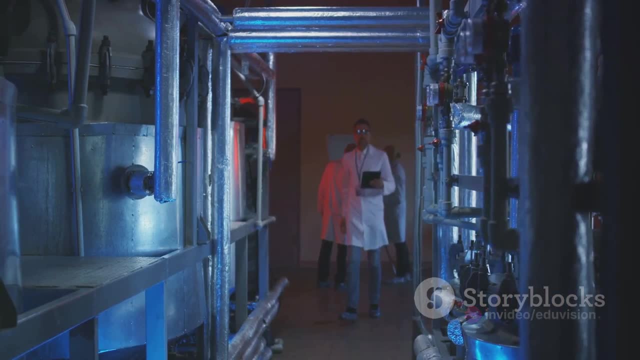 but what makes it so special? Bose-Einstein condensates have some truly mind-boggling properties. Now let's dive into the fascinating characteristics of Bose-Einstein condensates, or BCs for short. These are a state of matter that exists at extremely low temperatures. 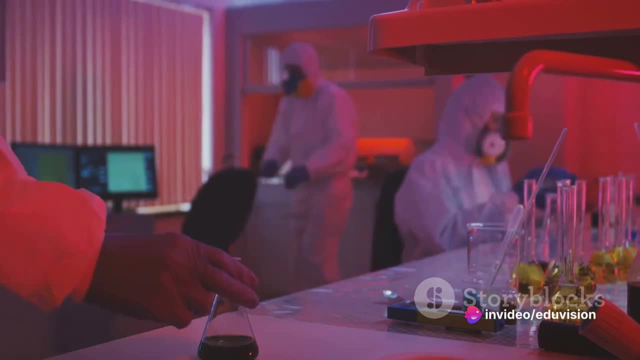 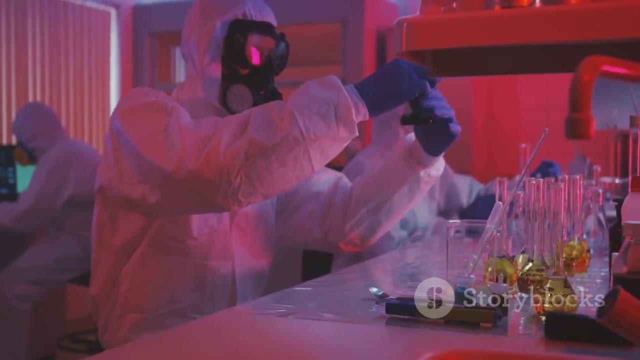 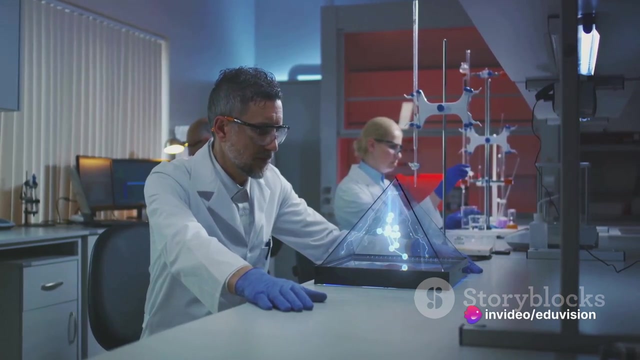 close to absolute zero, where the rules of quantum mechanics start to take precedence over classical physics. One of the most intriguing properties of BCs is super fluidity. This is a phenomenon where liquid, in this case a BC, flows without friction. Imagine a viscous liquid like honey. now picture it flowing as freely as water. 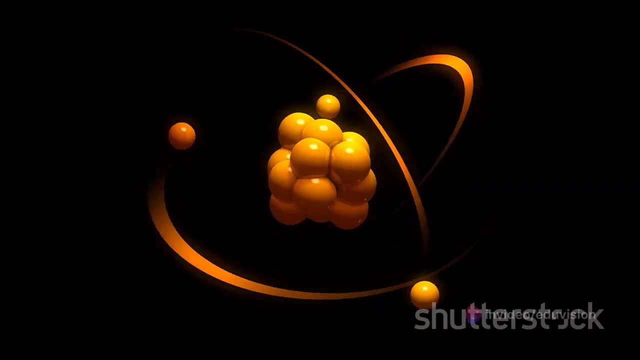 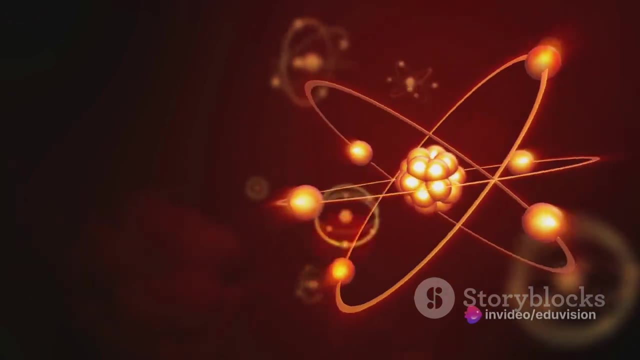 with no resistance whatsoever. That's super fluidity. for you. In a BC, atoms move in unison, behaving more like a single giant atom rather than individual ones. This coherence leads to the super fluidity we observe. Next, let's talk about matter wave interference. You might remember. 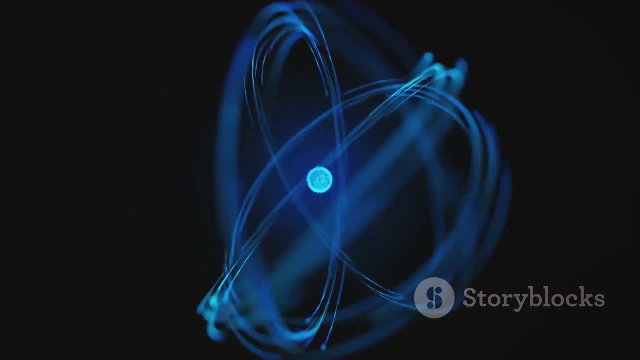 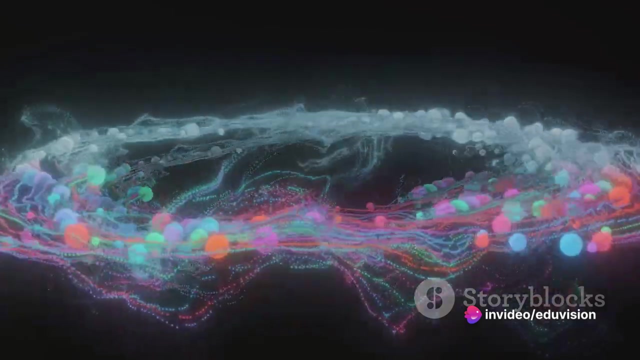 from quantum mechanics that particles like atoms can behave like waves. In a BC, the wave nature of atoms becomes more pronounced due to their coherence. When two BCs overlap, they create an interference pattern, much like how overlapping waves in a pond create a pattern of peaks and 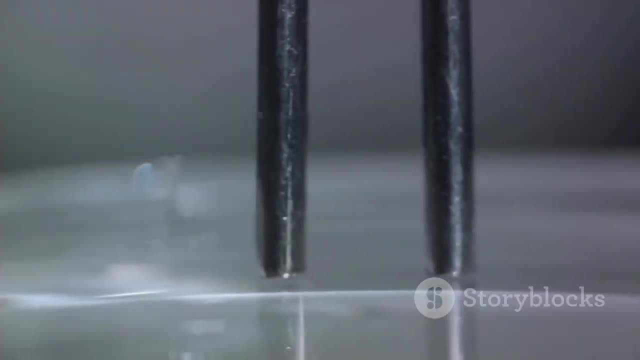 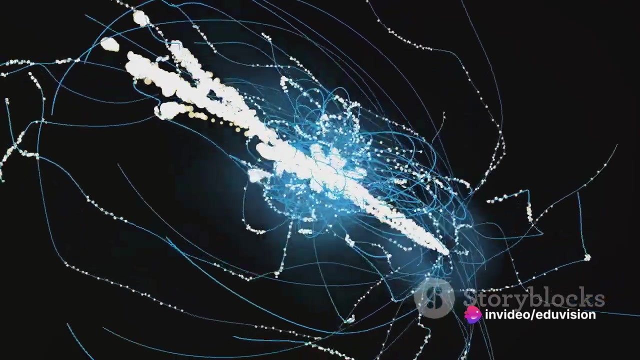 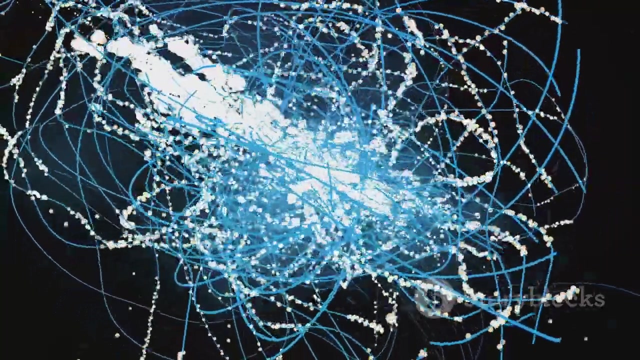 troughs. This phenomenon, known as matter wave interference, is a clear demonstration of the wave particle duality concept in quantum mechanics. BCs also exhibit extremely low entropy, meaning they are highly ordered systems. This is because at near absolute zero temperatures, the atoms have very little thermal energy to move around randomly. They instead occupy the lowest possible energy. 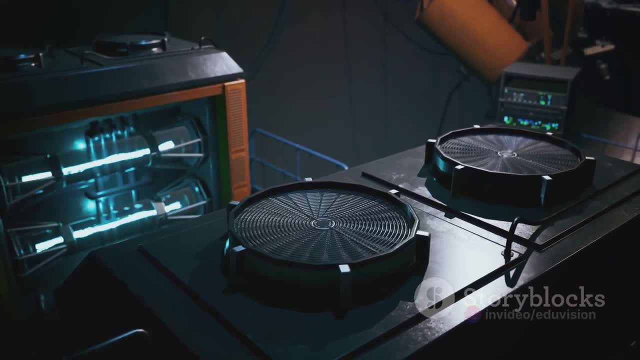 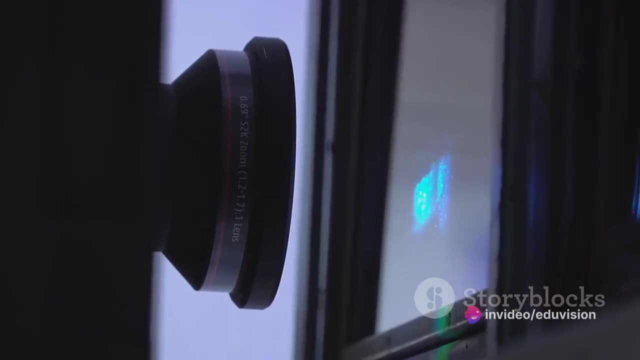 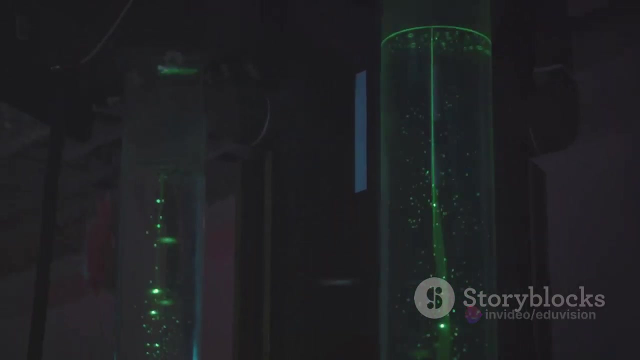 state, resulting in a state of high energy. And finally, BCs are incredibly sensitive to external disturbances. This makes them excellent for precision measurements, such as in atomic clocks or in detecting slight variations in gravitational fields. Those are some intriguing characteristics, but how does one create a Bose? 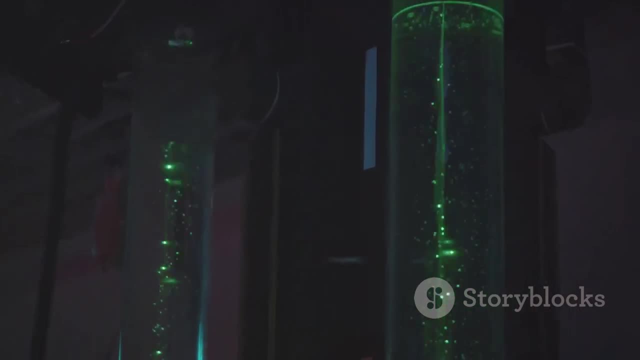 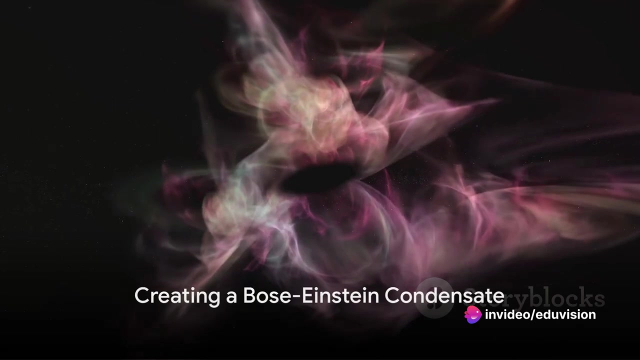 Einstein condensate. Stay tuned as we delve into the fascinating process of creating these extraordinary states of matter in the next scene. Creating a Bose. Einstein condensate is no easy feat. It's a little like trying to catch a snowflake in the Sahara. 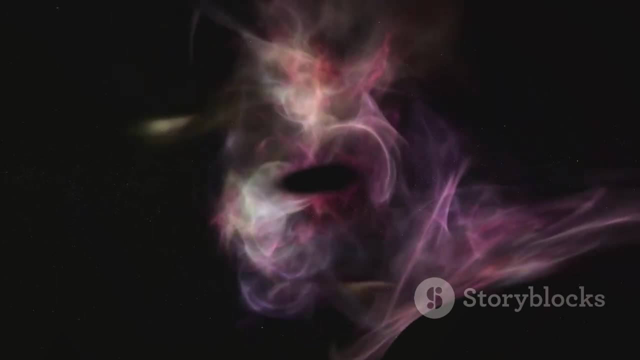 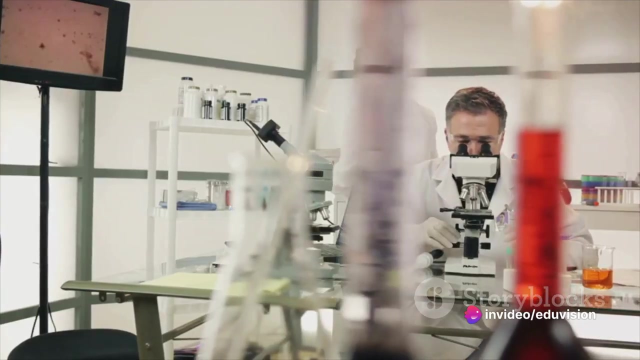 Or finding a needle in a haystack, But with a lot more lasers and magnetic fields To create a Bose, Einstein condensate or BC. scientists start with a cloud of atoms trapped in a magnetic field. This isn't your everyday cloud. it's a cloud of supercooled atoms. 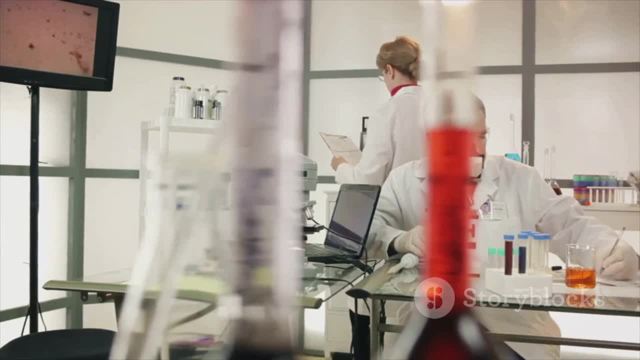 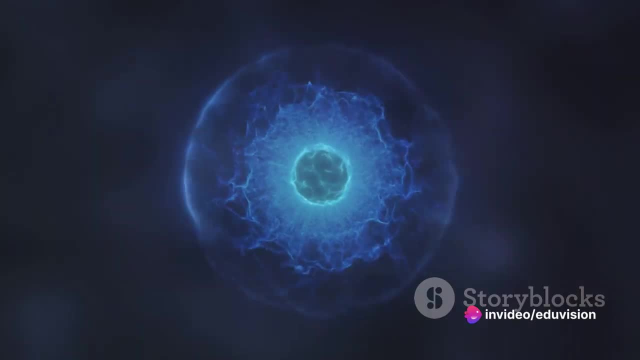 kept at a temperature colder than in the deepest depths of outer space. Next come the lasers. and no, these aren't your typical laser pointers. These are specially tuned lasers that are used to slow down the atoms. It's a bit like using a water hose to slow down a. 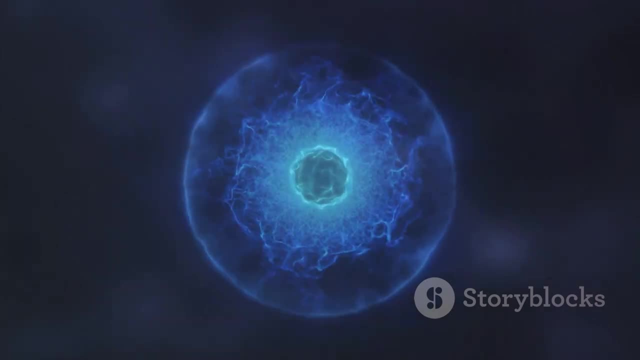 speeding car. The lasers are used to slow down the atoms. The lasers are used to slow down the atoms. The lasers are used to slow down the atoms. It's a bit like using a water hose to slow down a speeding car. The lasers bombard the atoms from all sides, causing them to lose energy and slow down. 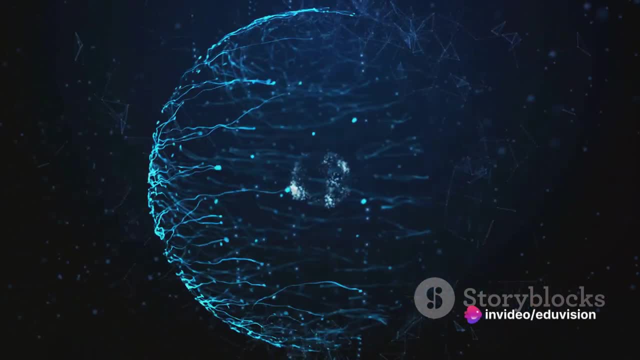 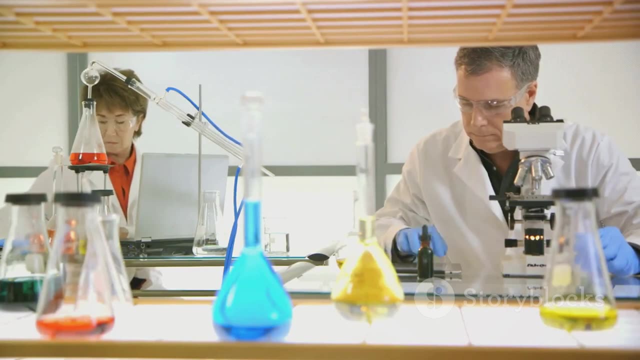 This cooling process is known as laser cooling, And it's one of the key steps in creating a BEC. but even after the laser cooling, the atoms are still not cold enough. That's when a second process called evaporative cooling comes into play. It's similar to how a 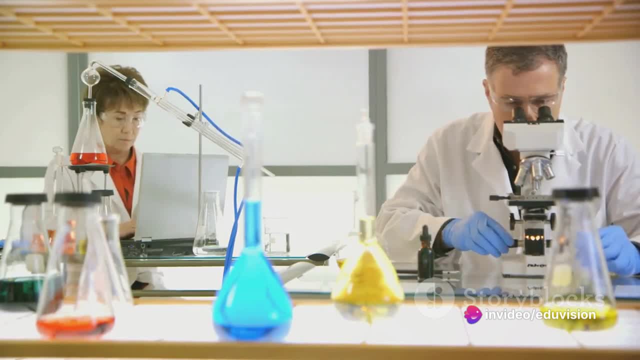 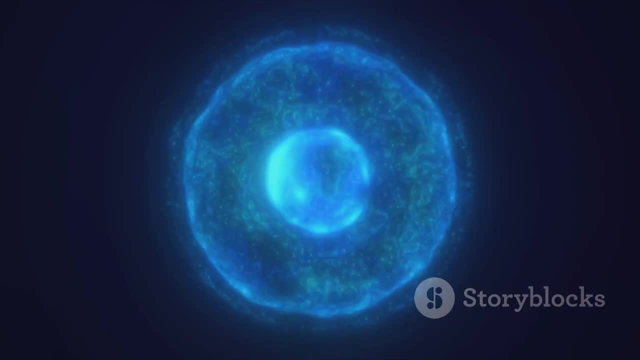 cup of coffee cools down. The hottest atoms are allowed to escape, leaving behind the colder ones. This process is repeated until the remaining atoms are so cold they're just a hair above absolute zero. This process is repeated until the remaining atoms are so cold they're just a hair above absolute zero. 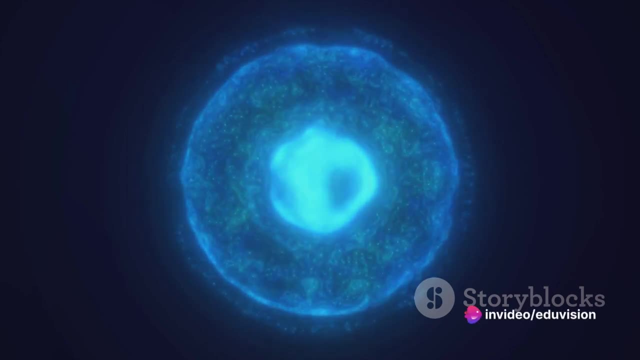 Now here's the magic: When the temperature gets this low, something extraordinary happens: The atoms start behaving like waves rather than individual particles. They overlap and become indistinguishable from one another, forming a single entity known as a Bose-Einstein condensate. 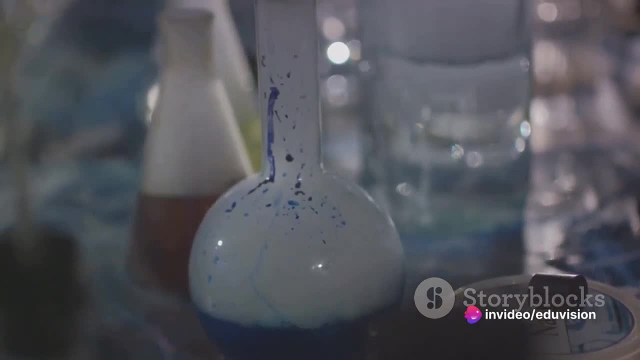 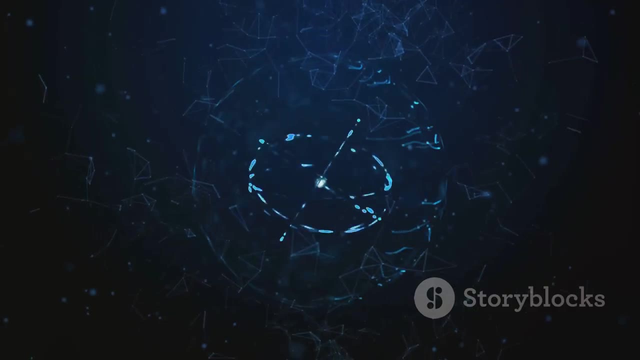 It's a state of matter that defies our everyday understanding of the world and brings us a step closer to the weird and wonderful realm of quantum mechanics. Creating a BEC is a complex and delicate process. It requires precise control over the environment and the careful manipulation of atoms. but the 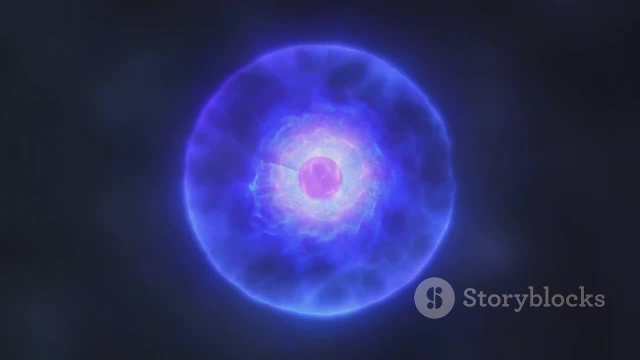 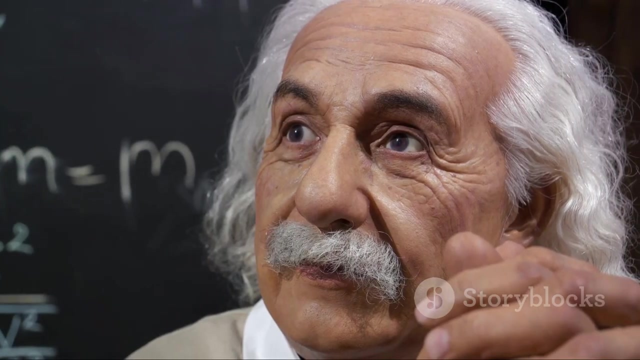 rewards are worth it. The BEC provides a window into the quantum world, and the potential applications are as exciting as they are vast, And that's how we get to see this fascinating state of matter. So there you have it, the Bose-Einstein condensate. We've dug deep into this fascinating state of 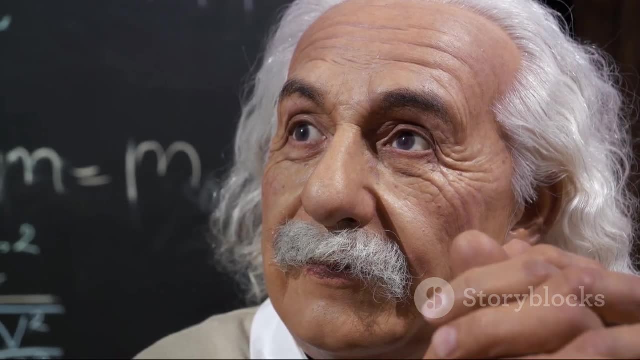 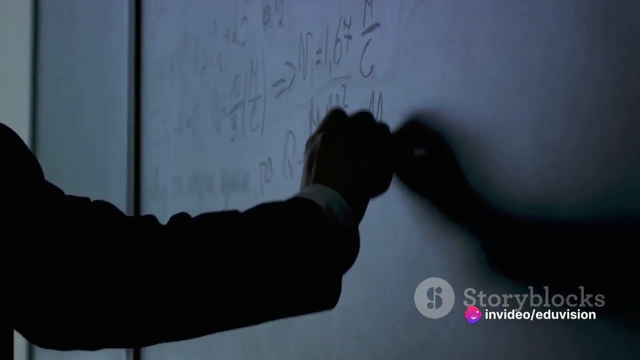 matter, from its inception in the minds of Satyendra Nath Bose and Albert Einstein, to its unique characteristics that set it apart from solids, liquids and gases. We've discussed the eerie, superfluid property where friction seems to vanish and the condensate flows without resistance. 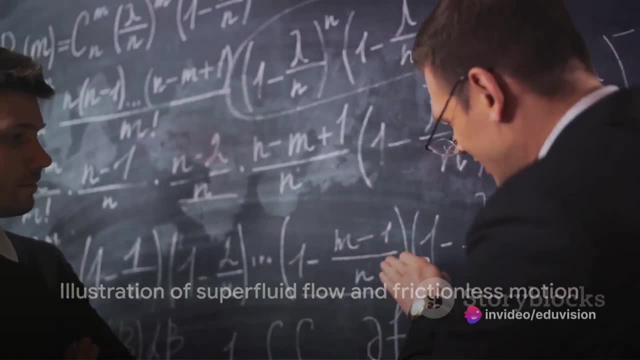 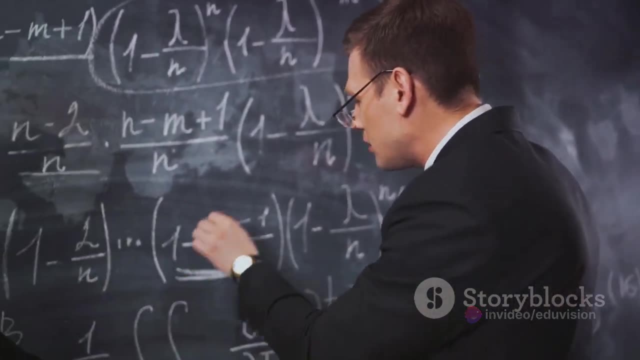 We've also touched on how it can be used to slow down light, a phenomenon that challenges our everyday understanding of the universe. Creating a Bose-Einstein condensate with temperatures colder than those found in outer space is no small feat. It's a testament to the stunning 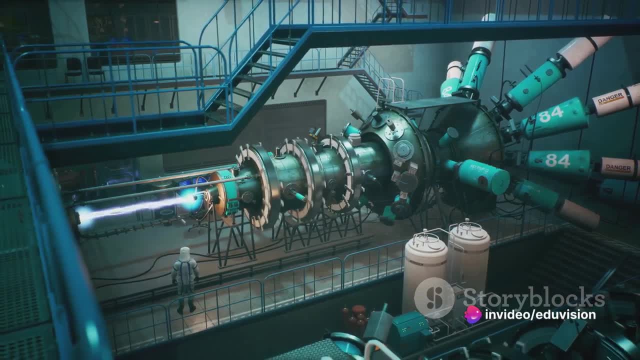 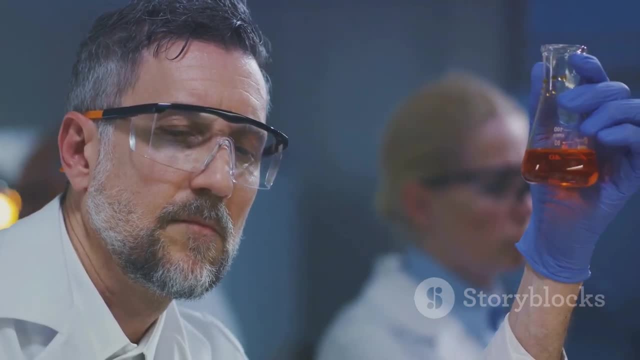 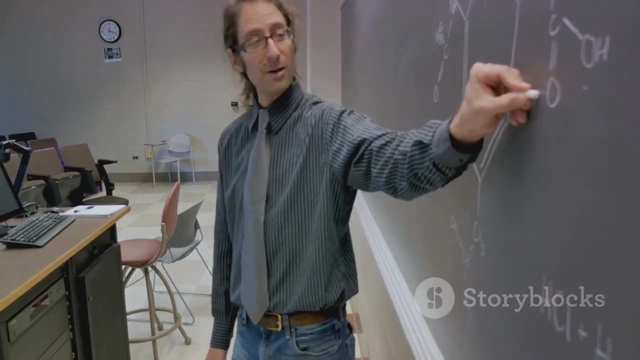 advances in science and technology, But our journey doesn't end here. There's so much more to learn and discover about BECs. so keep that curiosity burning, keep asking questions and never stop exploring the fascinating world of quantum physics. Remember, in the world of quantum physics things can get really cool.